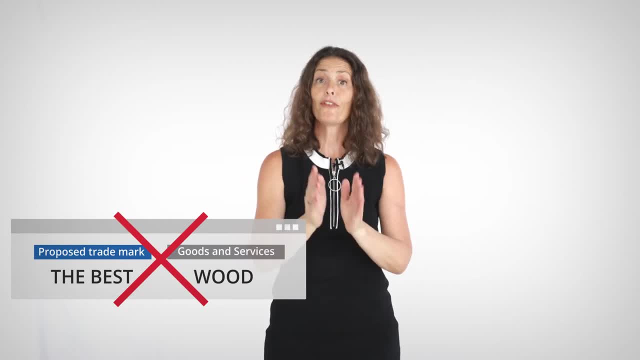 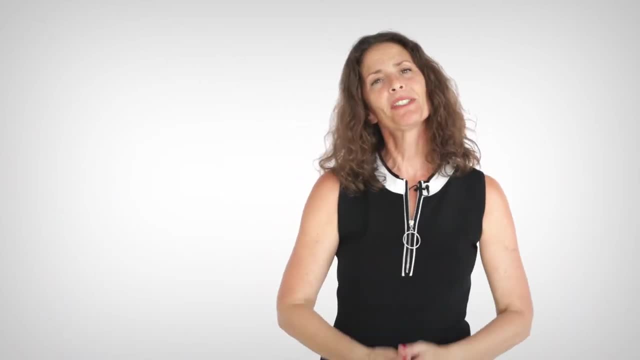 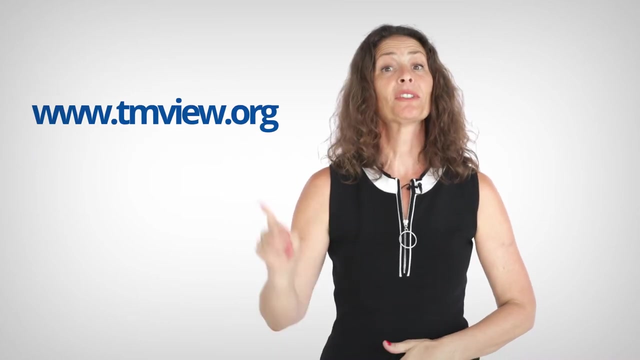 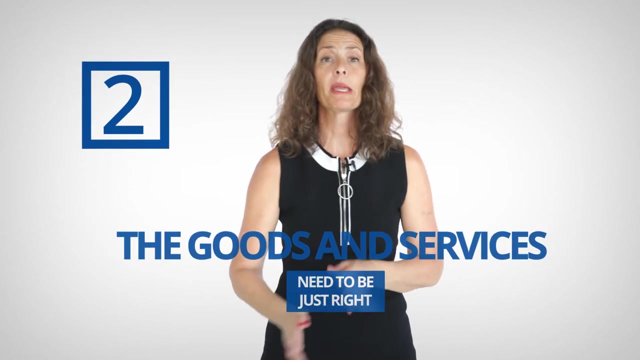 distinctive when it describes what you sell. So first check on our website if your mark meets the criteria. Also, your new mark must be different from those already registered. To check if there are marks identical or similar to yours, go to TMview and do a pre-screening search. The second most common mistake is when 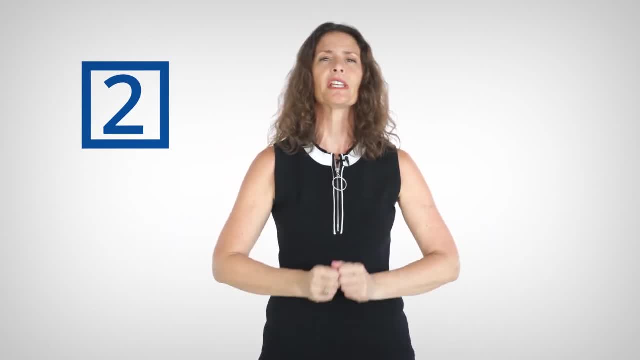 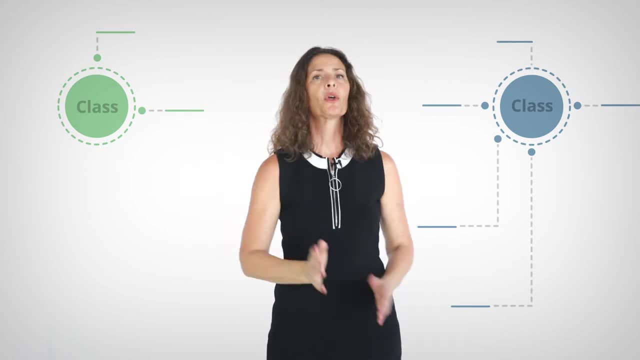 people mess up the list and goods and services they choose for the EUTM to cover. They should be just right: Not too few, not too many, not too long. When you apply for an EUTM, the basic application fee covers one class, So what you need to. 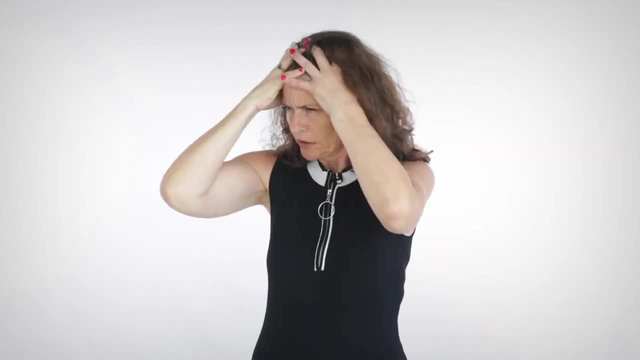 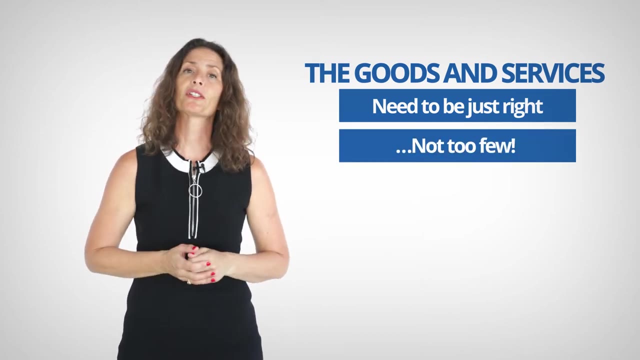 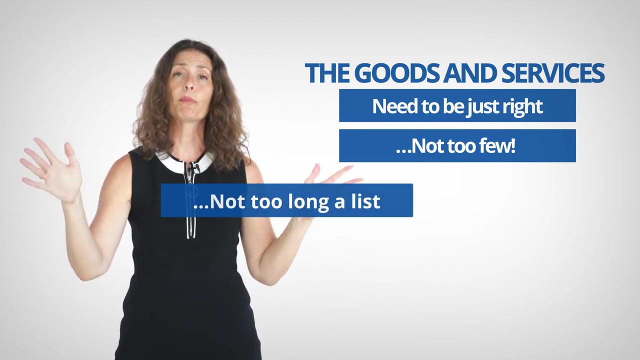 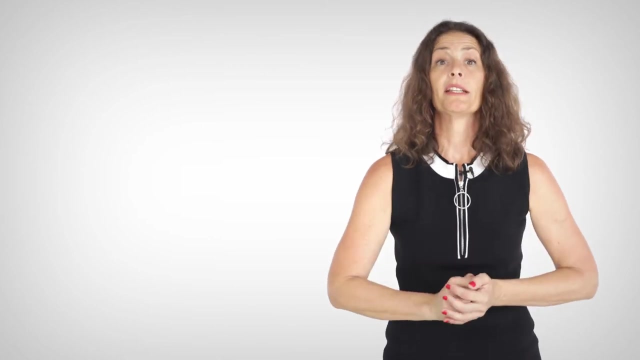 is. be realistic and think You cannot add goods or services after the application or registration. so think about what you're going to sell now and within a foreseeable future. But if you have a very long list or you put down too many classes, then you may put your trademark at risk. Remember that an EUTM 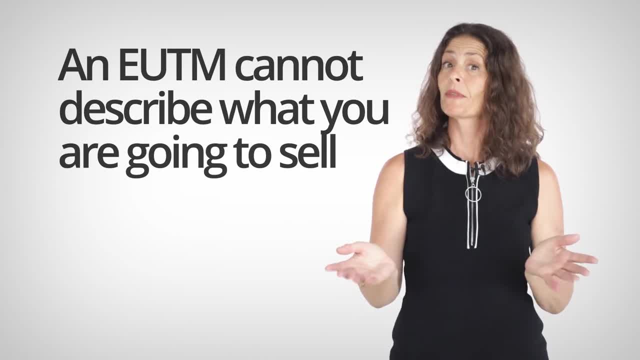 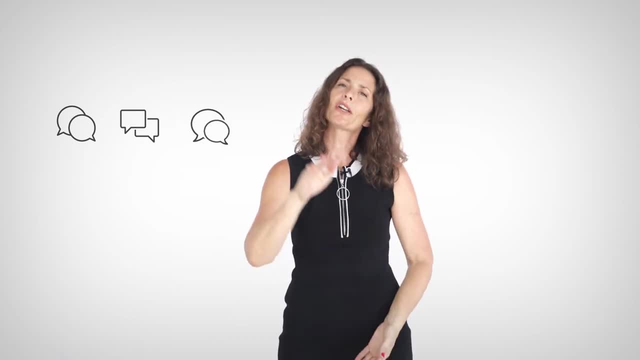 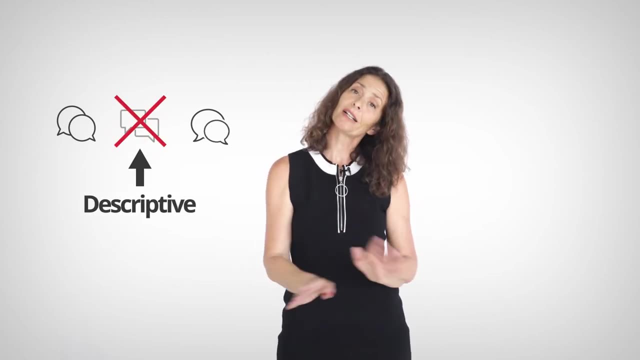 cannot describe what you're going to sell. Well, the EUIPO examines the trademark in all of the EU official languages, So the longer your list is, the bigger the risk is that your mark will be descriptive in one of those languages and that the mark cannot be registered, Also with a very large scope. 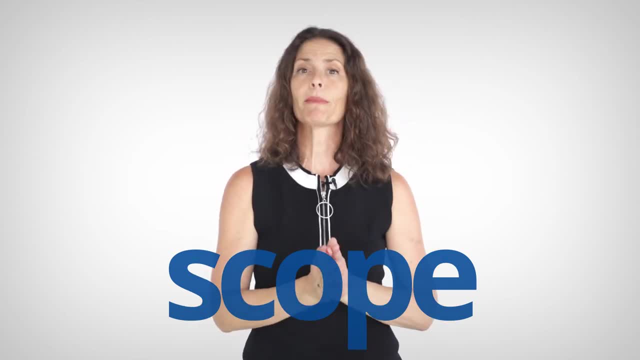 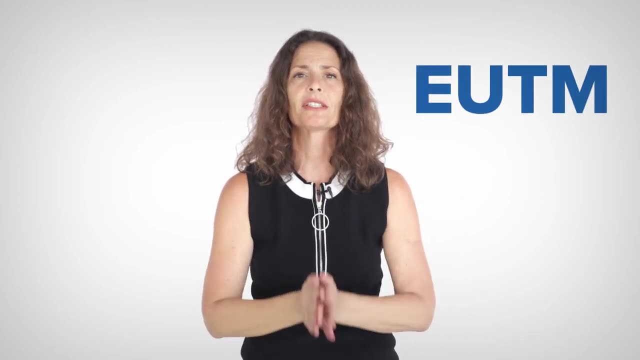 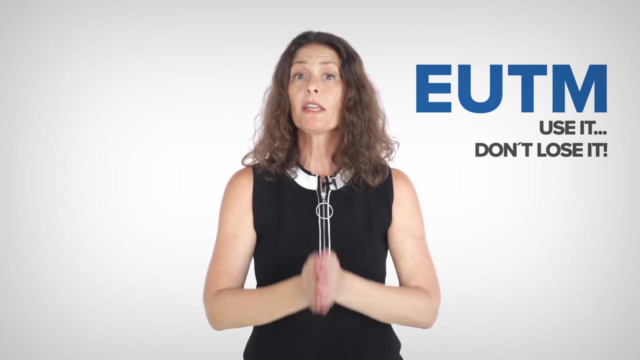 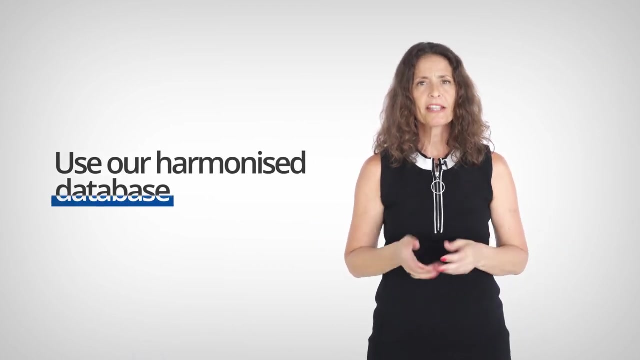 the risk that other companies with similar trademark will oppose your mark is bigger, And if you don't use the EUTM for the goods and services that you have registered for in the first five years, you risk losing some of those or even the trademark itself. So a good tip is to use our database to select your goods. 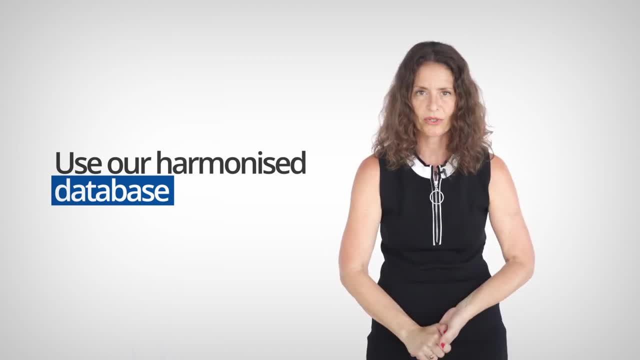 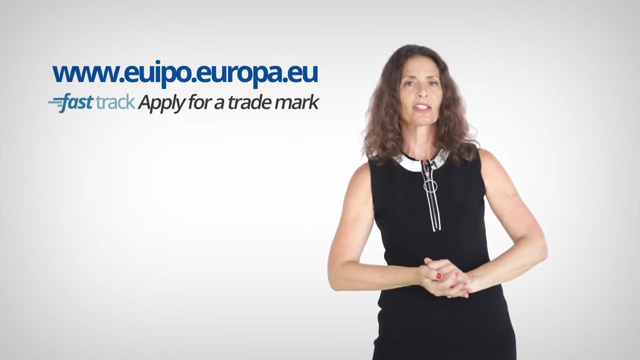 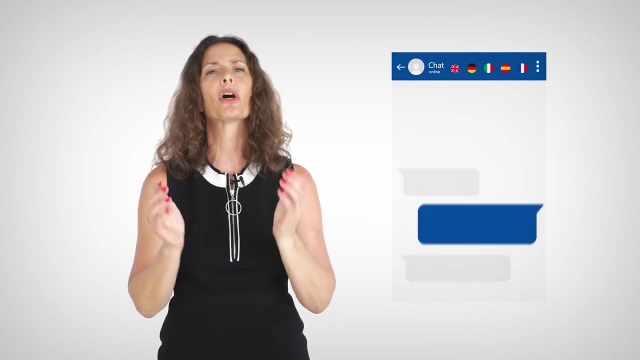 and services to avoid errors in the registration process. This tool is available for you automatically when you use our simplified fast-track trademark application from the website. If you do that, you can get your EUTM for free. You can also use the online chat to solve any doubts on the spot.